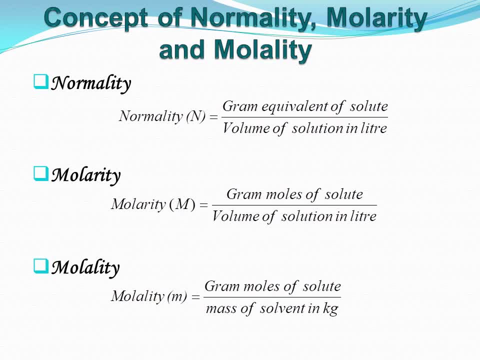 There are three ways of expressing the concentration of solution containing either solid or liquid solute, Namely normality, molarity and molality. First, we understand what is normality. Normality can be defined as the number of gram equivalents of solute dissolved in one liter of solution. 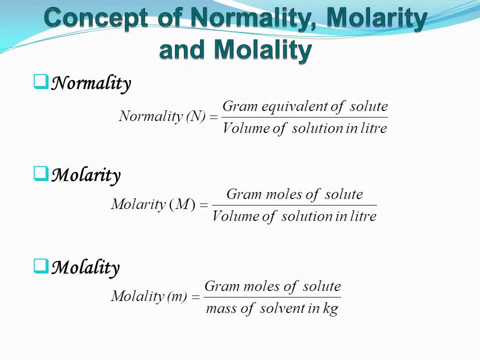 It is designated by the symbol N. Second, we understand what is molarity. It is defined as the number of gram moles of the solute dissolved in one liter of solution. It is designated by the symbol M. Third, we understand molality. 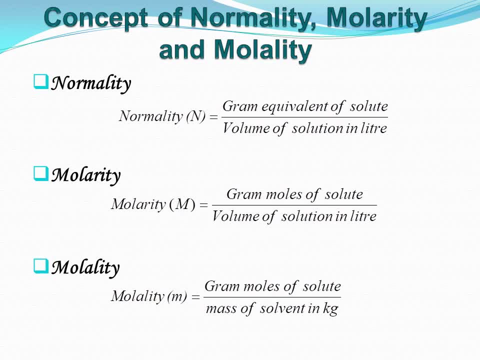 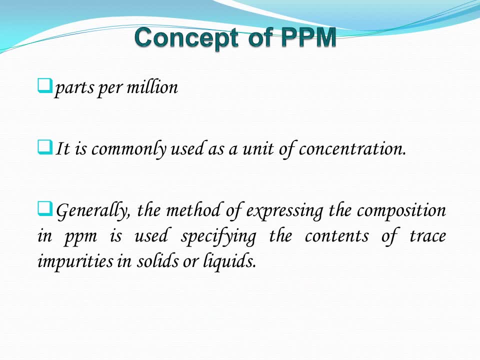 It is defined as the gram moles of the solute dissolved in one kilogram of solvent. Next we comes to the concept of PPM. It is the short form of parts per million, That is, parts of one substance present in million parts of another substance, especially solvent. 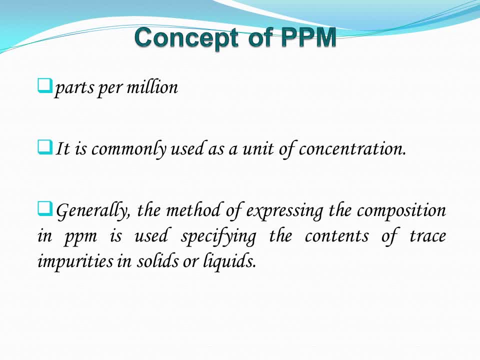 It is commonly used as a unit of concentration. Concentration may be defined as the amount of solute present in known amount of solvent. Generally, the method of expressing the composition in PPM is used, specifying the contents of present impurities in solids or liquids. 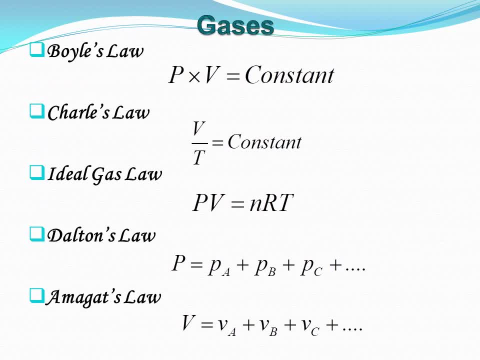 Now we understand some laws applicable for gaseous state. While dealing with substances existing in the gaseous state, the relationship among the temperature, pressure, mass and volume must be known. First we take Boyle's law. According to Boyle's law, for a given mass of an ideal gas, the product of the pressure and volume is constant at a constant temperature. 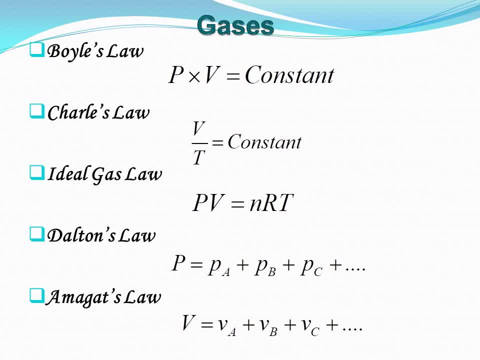 That is P into V equals to constant. Next is Charles' law. According to Charles' law, for a given mass of an ideal gas, the ratio of the volume to temperature is constant at a given pressure. That is, V by T equals to constant. 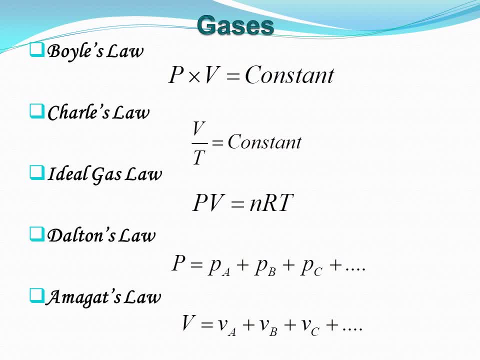 On combining these two laws, we get the expression for an ideal gas law, as PV equals to nRT, where R is the universal gas constant and n is the number of moles. Next is Dalton's law, which states that the total pressure exerted by the gaseous mixture is equal to the sum of the partial pressures of component gases. 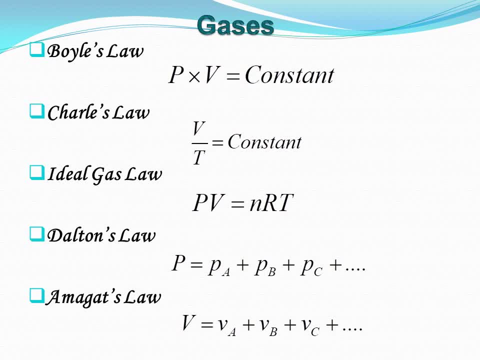 That is, P equals to pA plus pV, Where p is partial pressure, which is the pressure in the mixture of gases that would be exerted by that component gases if they were present in the same volume and temperature. Next is Amaget's law. 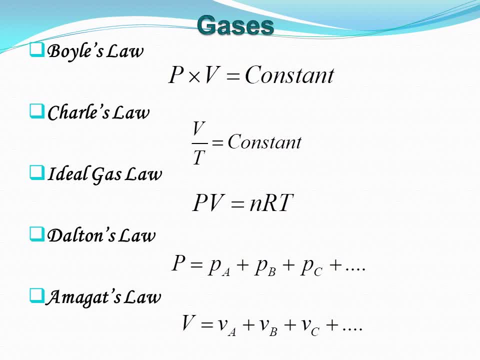 It states that the total volume occupied by the gaseous mixture is equal to the sum of the pure component volumes, That is, capital V equals to small vA plus vB plus small vA, Where small v is pure component volume, which is the volume that would be occupied by that component gases if they were present at the same pressure and temperature as the mixture. 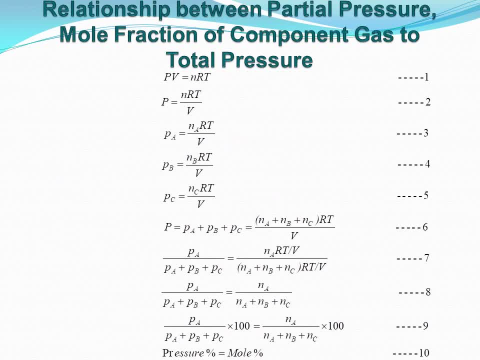 Then comes the relationship between partial pressure and mole fraction of component gases in total pressure. The composition of component gases present in gas mixtures is generally expressed in the following way: In case of gas mixtures containing in closed vessels, the molecules of each component gases are distributed throughout the entire volume of the container. 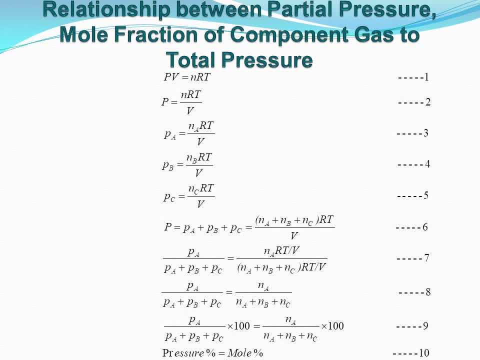 The total pressure exerted by the entire mixture is equal to the sum of the pressures exerted by each component gas. From the ideal gas law we know that pV equals to nRT. On rearranging this equation we get p equals to nRT by V. 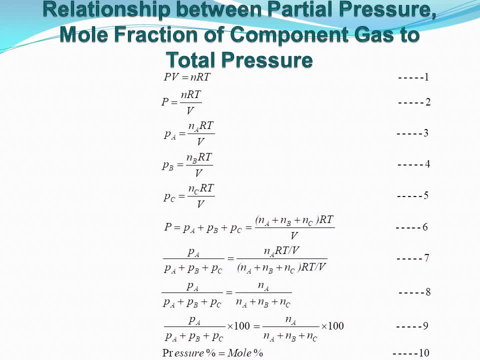 Writing this equation in terms of different components- gases- we get p equals to nRT by V. Similarly, p equals to nRT by V And p equals to nRT by V. Applying these three equations, adding these three equations, we get: 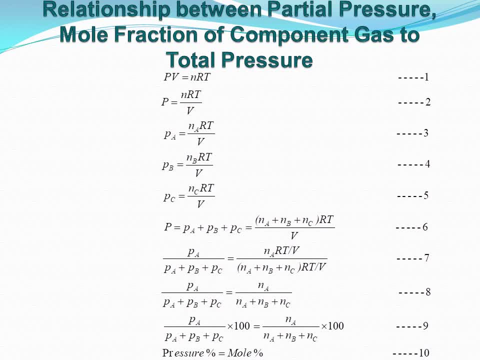 capital. P equals to small pA plus pB plus pC equals to nA plus nB plus nC into R, into T, divided by V. Dividing equation 3rd by equation 6, we get pA divided by pA plus pB plus pC equals to nA into RT divided by V, whole divided by nA plus nB plus nC into RT by V. 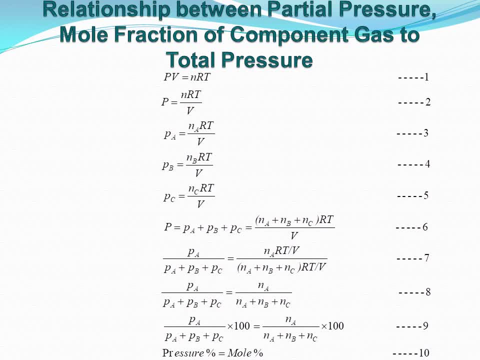 On simplifying above equation: we get pA by pA plus pB plus pC equals to nA by nA plus nB plus nC. Multiplying both sides of this equation by 100, we get pA by pA plus pB plus pC into 100 equals to nA by nA plus nB plus nC into 100. 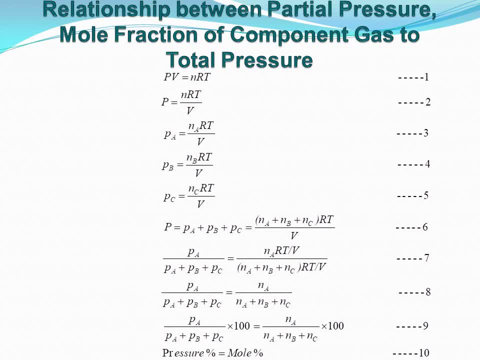 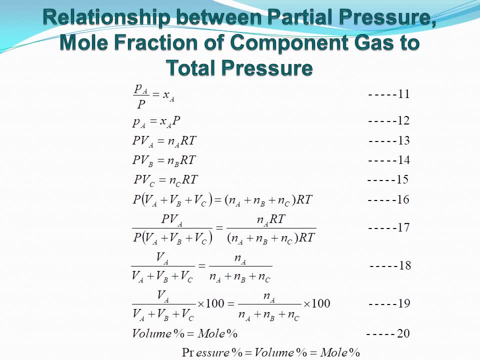 That is, pressure percent equals to more percent. From equation 8, we get pA by P equals to x. On rearranging, we get pA equals to x into P When ideal guess was applicable. it can be written for guess components A, B and C as: 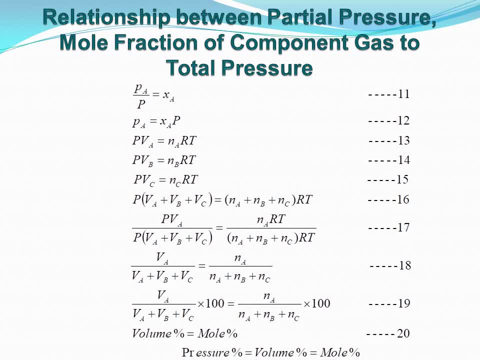 p into VA equals to nA into RT. Similarly, p into VB equals to nB into RT and p into VC equals to nC into RT. Adding above three equations, we get p into VA plus VB plus VC equals to nA plus nB, plus nC into R, into T. 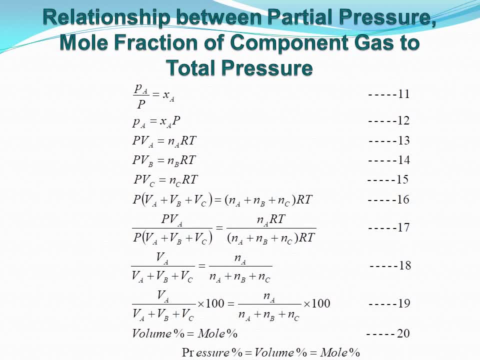 Dividing equation 13 by equation 16, we get p into VA divided by nA plus nB plus nC into R into T, d into VA. divided by p into VB plus VB plus VC equals to nA into RT. divided by nA plus nB plus nC into RT. 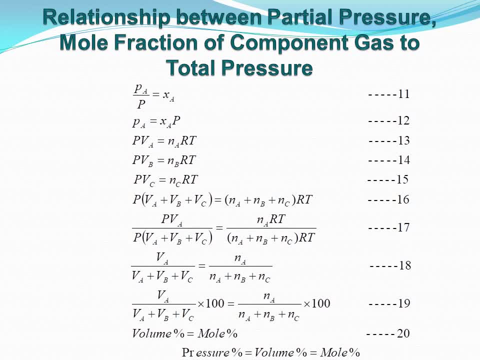 On rearranging this equation, we get vA by VB plus VB plus VC equals to nA divided by nA plus nB plus nC. Multiplying both sides of this equation by 100, we get vA by VB plus VC into 100. 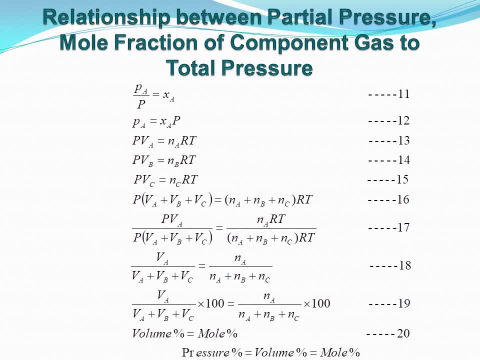 equals to nA by nA plus nB plus nC into 100.. That is volume percent equals to mode percent. Combining equation 10 and 20, we get pressure percent equals to mode percent. equals to volume percent. Then we comes to. 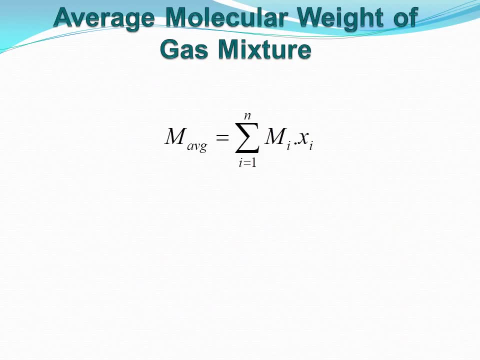 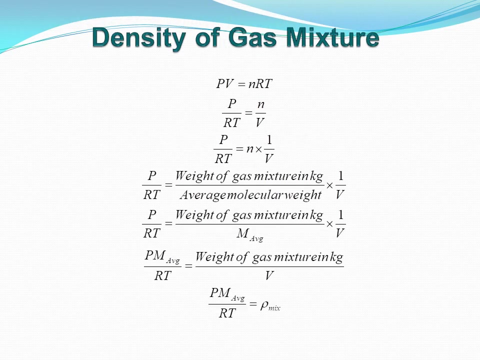 average molecular weight of gas mixture. It is the sum of the product of molecular weight and mode fraction of component gas. It can be expressed as: M. average equals to summation. i equals to 1 to n. Mi into Xi. Then we comes to. 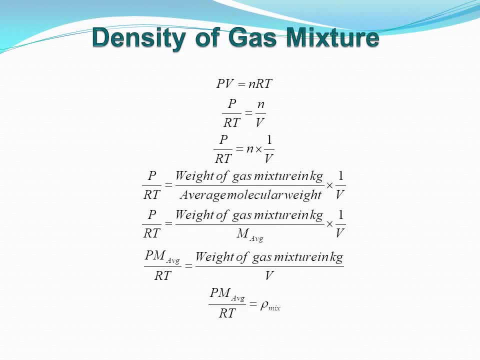 density of gas mixture. It can be easily calculated by the use of ideal gas law at a given temperature and pressure of the gas mixture. For calculating the density one must know the average molecular weight of the gas mixture. From the ideal gas law we know that 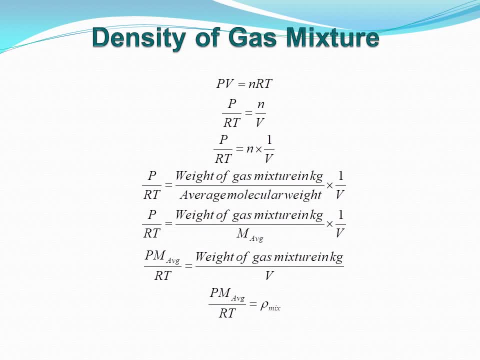 PV equals to nRT or we can say that P by RT equals to n by V. It can be written as: P by RT equals to n into 1 by V, Where n can be replaced. and written as: the ratio of weight of gas mixture in kg. 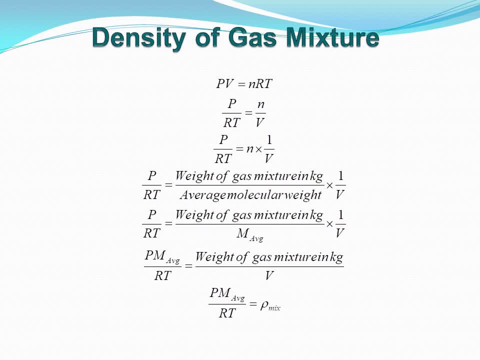 divided by average molecular weight. Then, in short, average molecular weight can be written as M into average, M average. Therefore the equation becomes PM. average by RT equals to weight of gas mixture in kg divided by V. The ratio on right side is known as: 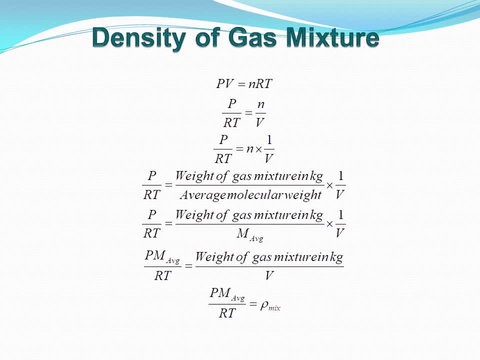 the density of the gas mixture. Therefore we can write P into M. average by RT equals to rho mix, Where rho mix is the density of the gas mixture, which is equals to pressure, into average molecular weight divided by R into temperature. Next is non-ideal behavior of gases. 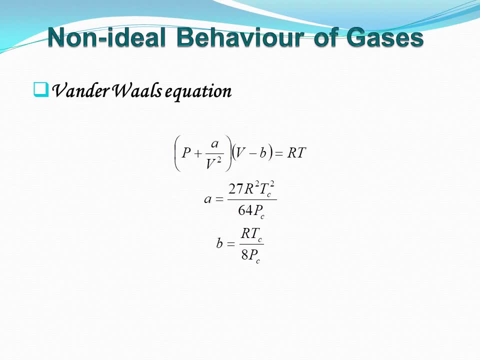 In order to account for non-ideal behavior of gases, Wender was proposed an equation of state as P plus A by V square into V minus B equals to RT. The values of constant A and B depends on the gas and hence can be evaluated. 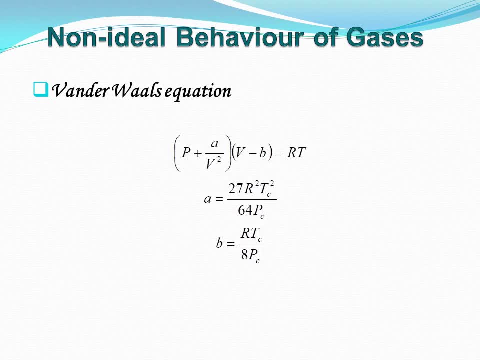 using the following equation: as: A equals to 27 into R square into T c square, divided by 64, into P p, and B equals to R into T c, divided by 8, into T c, Where T c and T c are critical pressure and temperature respective.